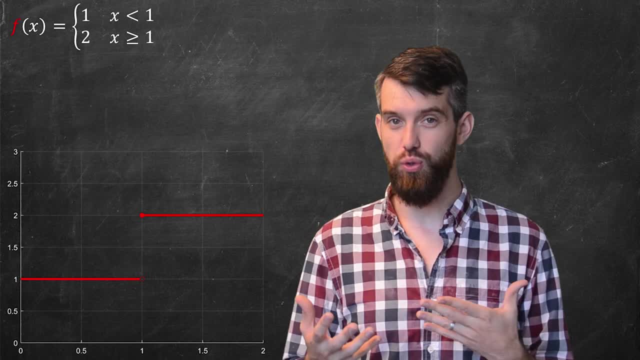 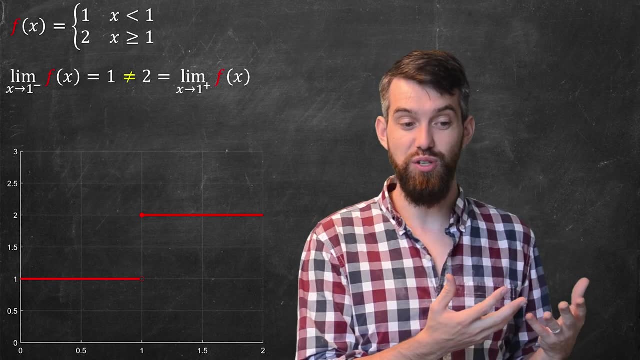 than 1, and it's the value 2 when x is greater than or equal to 1.. Well, in this case, we say the limit does not exist. Indeed, the limit from the left when x is less than 1, that's easy to. 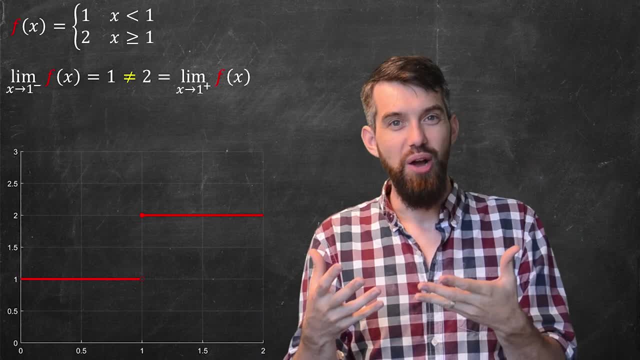 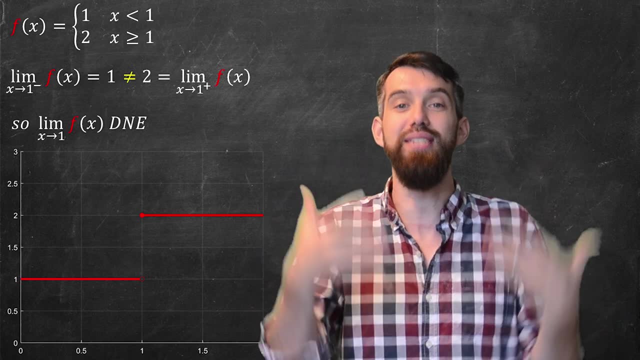 compute, That's just equal to the value of 1.. But the limit from the right, when x is greater than 1, this is equal to 2.. So the limit from the left and the right do not match and so we say the limit did not exist. However, in this different example where the 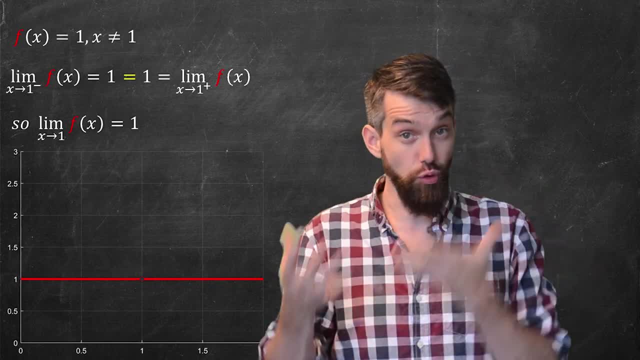 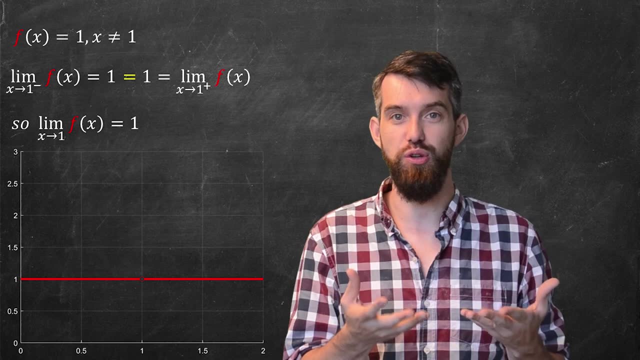 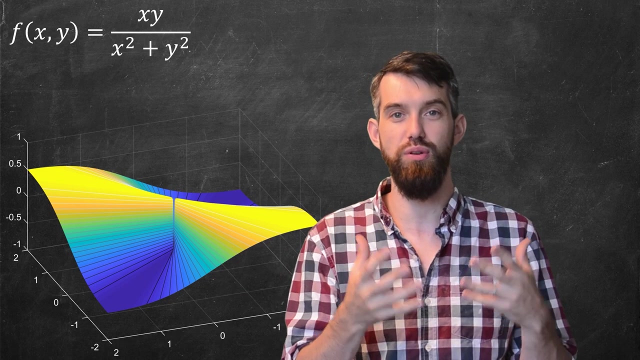 function is not defined at one point, but to the left and to the right, the function is indeed just equal to 1.. In this case, we said that the limit did exist and was equal to the value of 1.. So let's return to our multivariable case where we have this problem: spot the spot 0,. 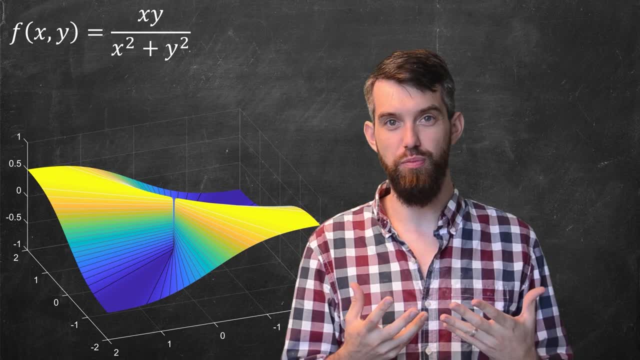 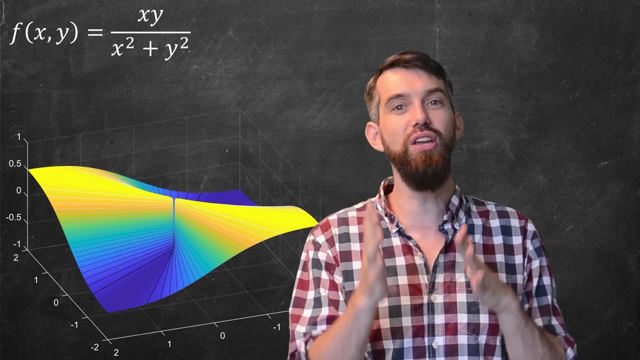 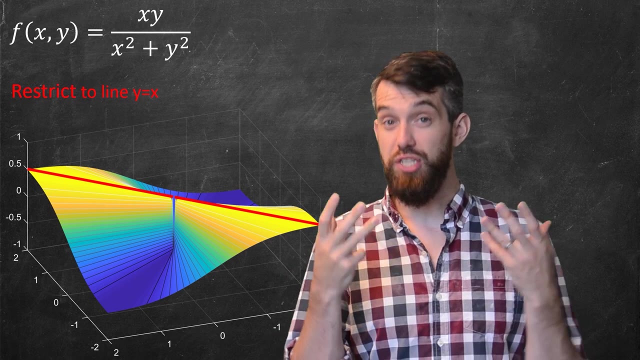 and we want to investigate the limit as I get close to that particular point. One way I can start to grapple with this problem is to restrict myself to a particular direction, a particular line. So let me demand that y is equal to x. This is a restriction and it's going to make. 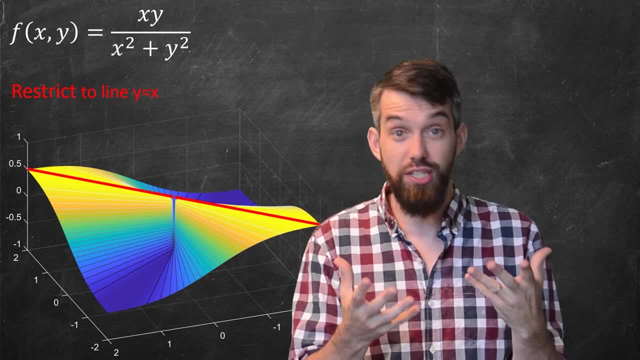 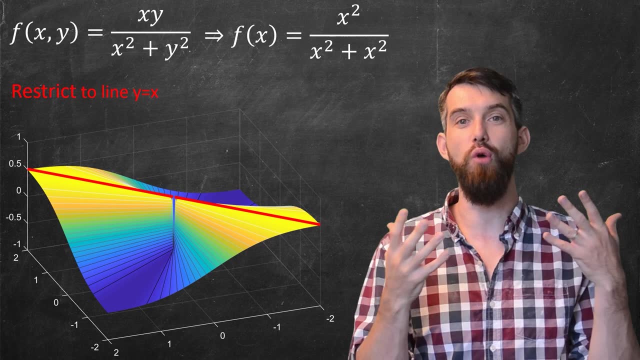 this multivariable function, just a single variable function, just in terms of x, that we know how to do. Indeed, everywhere there's a y, we come and plug the x value in and I'm just left with x squared over x squared. So I'm going to put in a x value and I'm going to put in a y value, and I'm 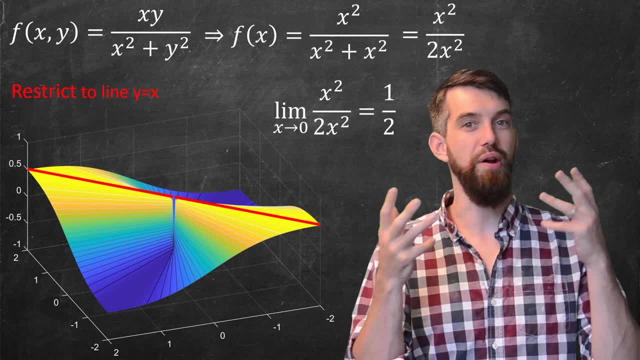 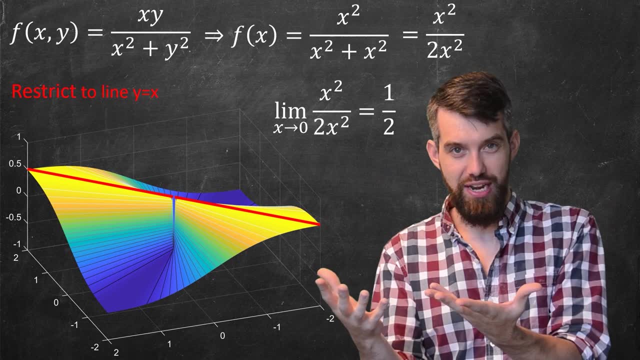 x squared over, x squared plus x squared, and then that's just x squared over 2x squared, which is one half. Now, the real strength of what we did is that I did not have to give you a new definition for what the limit meant in a higher dimensional context. I just put a restriction on, and then it. 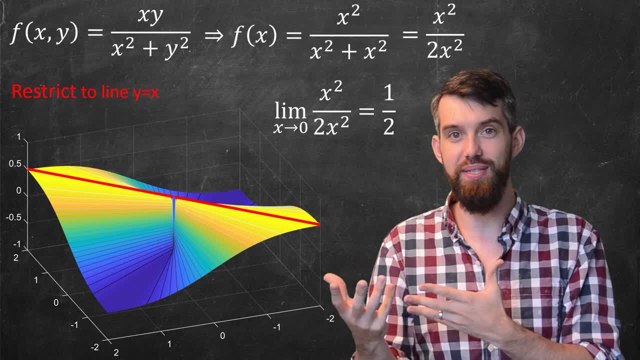 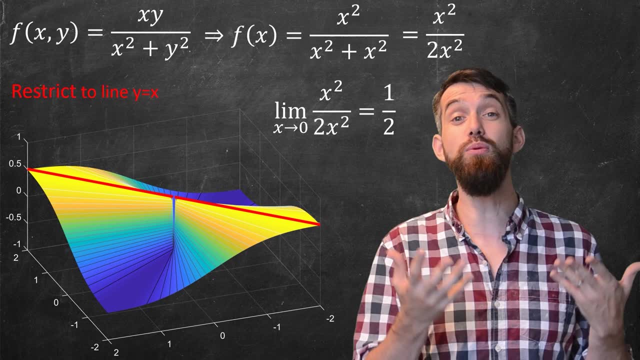 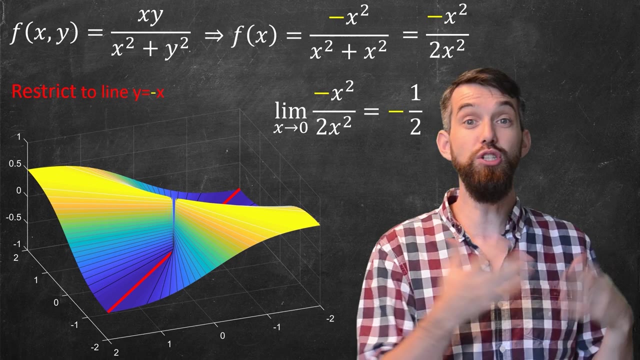 became the old one-dimensional concept of a limit and we computed this out. However, what if I changed my restriction? I don't have y equal to x. I impose, for example, y equal to minus x. Watch what happens. There's a graphical change and an algebraic change. Algebraically, the equation y equal to minus x. 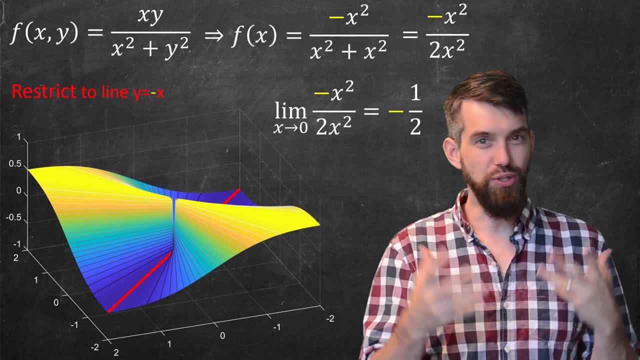 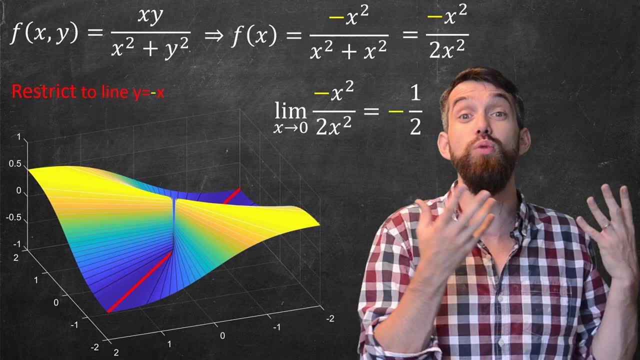 just means I get a whole bunch of minus signs everywhere through my calculation and the result of that is I get the value of minus one half for my limit. So along this line it's minus one half, whereas on the previous line it was plus one half. Now, graphically, what's happened? when I'm 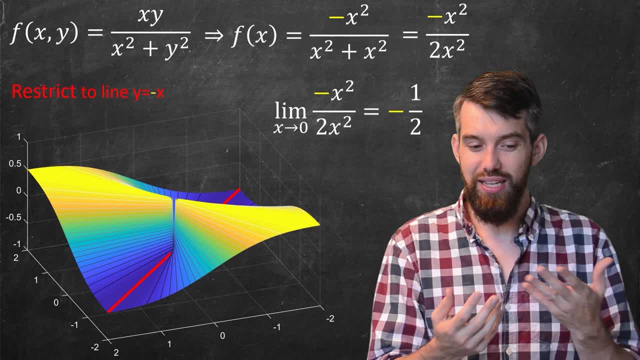 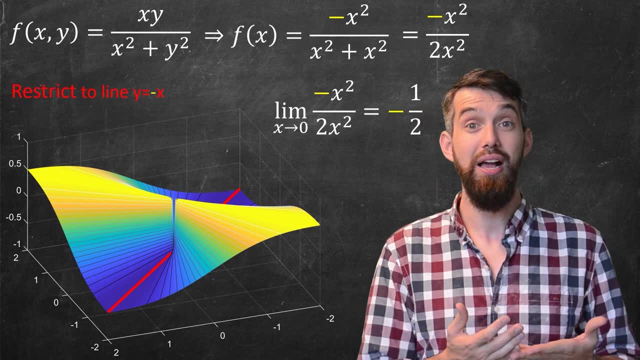 restricting myself. y equal to minus a half is now that I'm on a new line. the heights along that line are quite a bit different. They're much lower down than they used to. that's why we have this limiting value of minus one half, much smaller than it used to be for plus one half. 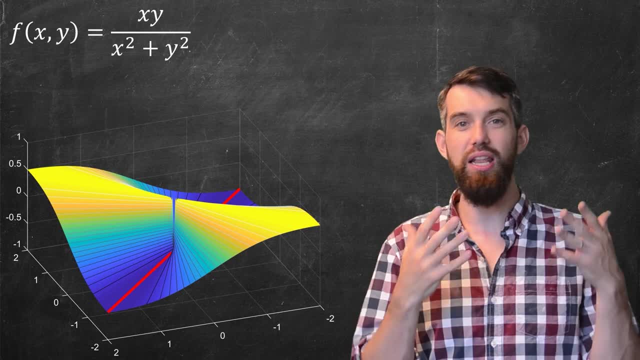 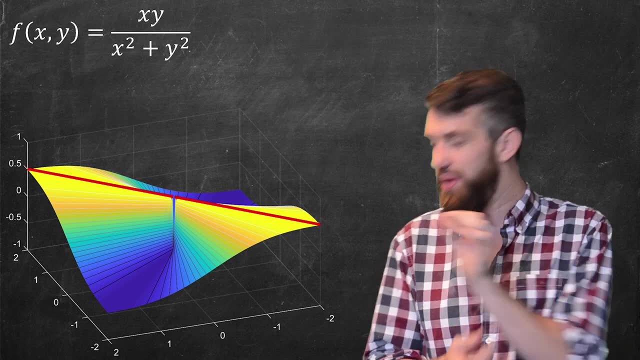 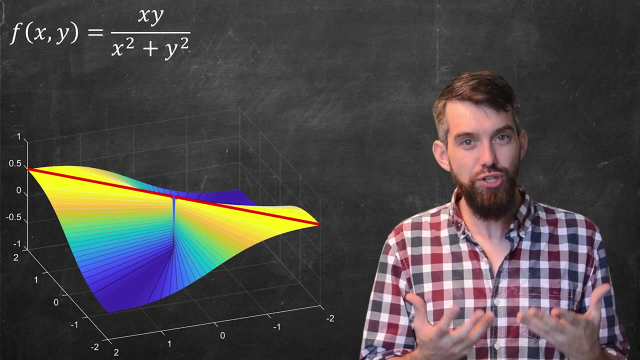 Indeed, if I focus just on that line, if I change that line from y equal to x to a bunch of different lines, what we see is that the limit, the spot in the middle where there's sort of a break in this particular function, there's this spot where it's undefined that that approach is closer and closer. 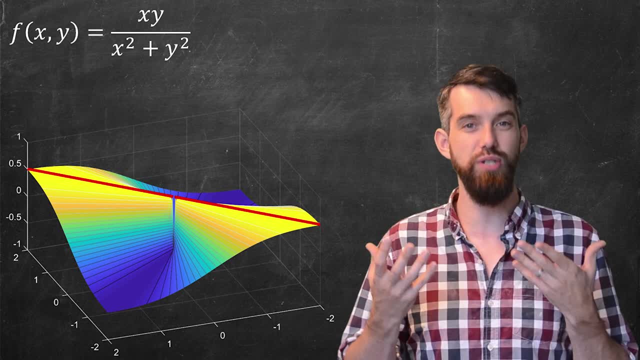 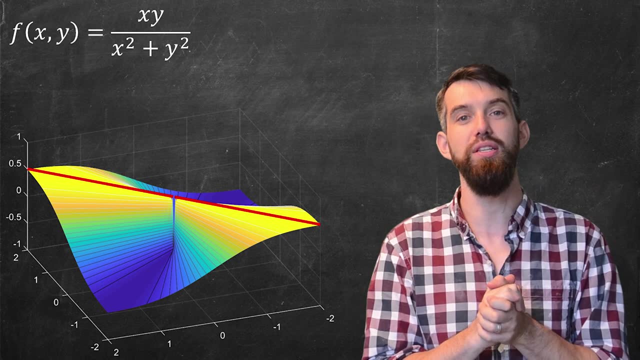 to a bunch of different values depending on the line you restrict it to. So what this makes me think is: So what this makes me think is is that there is no limit for this function, as x goes to the point when you approach on some lines. 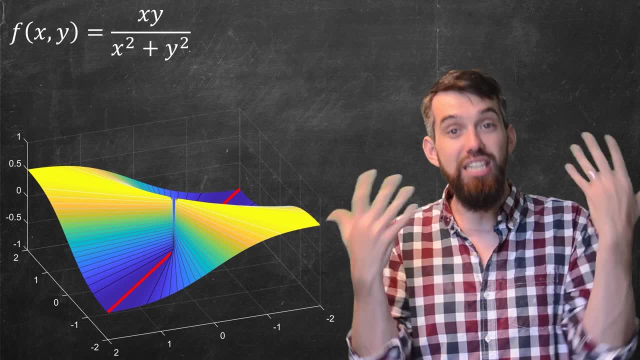 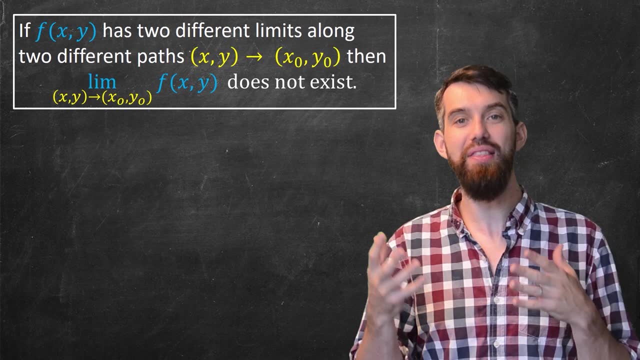 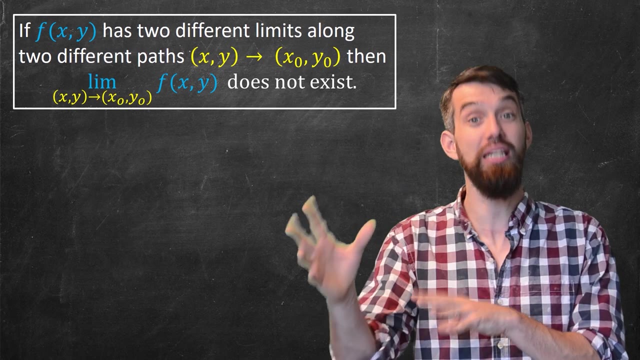 it looks like it's getting close to a value, but if you approach it in a different way, aka along a different line, then you get to a different value. this is called the two path test, for a limit not existing. it says that if you go along one path, then you get some particular limit of going along. 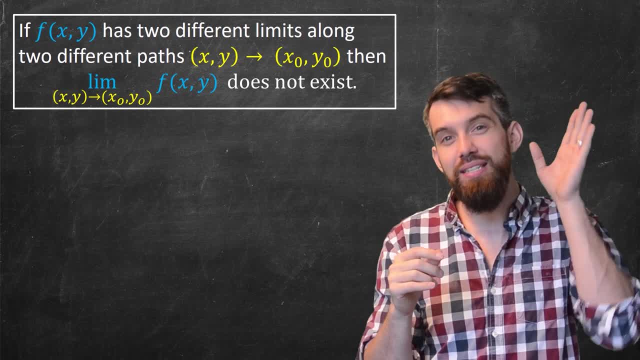 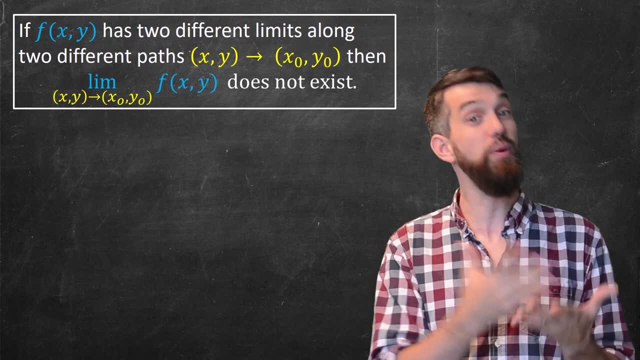 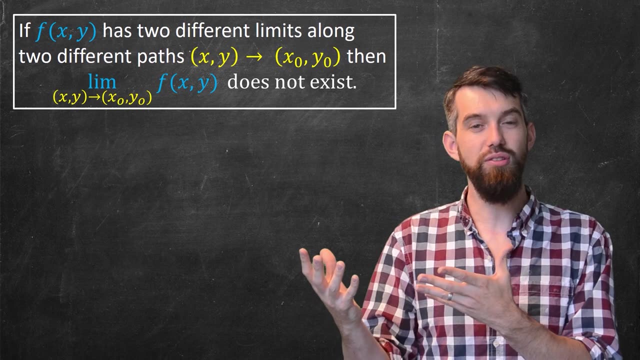 that one path and then you go along a different path and you get a different limit, then it says: for sure, the limit does not exist. now that leaves me with two questions that we need to take up in the future. now, this test only tells us when a limit does not exist. so the question is, if you go, 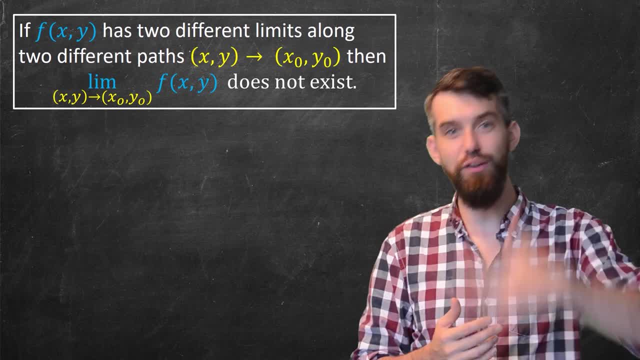 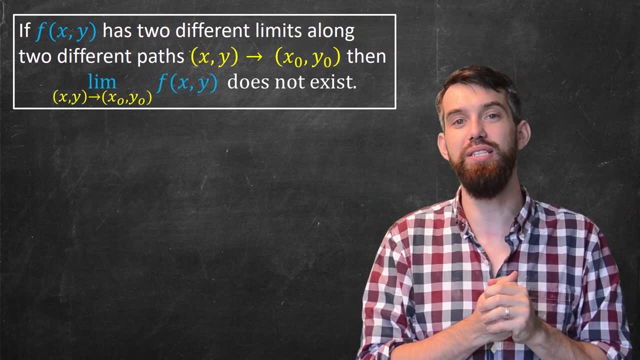 along one path- and it is a value- and go along a different path and a different path and a different path. they're always the same value. well, what exactly does a limit existing in the multi-variable context mean? that's the first question that we can think about for the future. 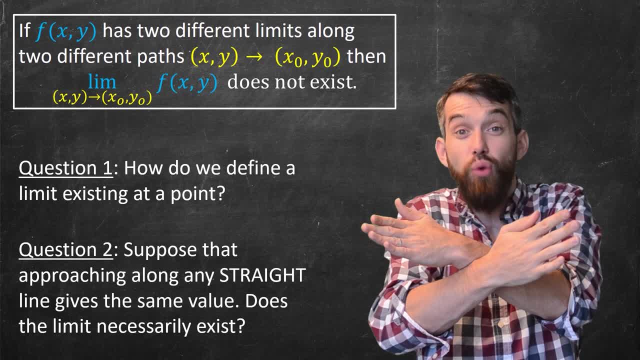 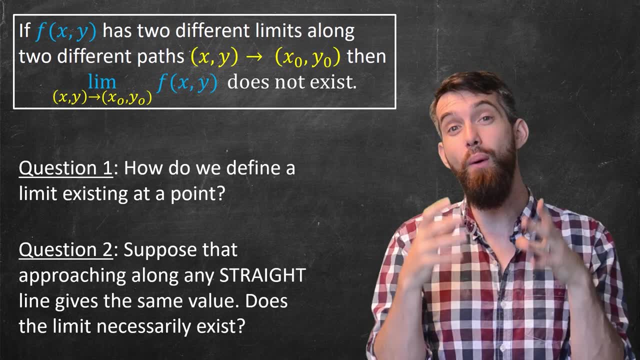 and then the second question says that i've been focusing on straight lines, different straight line paths, and perhaps it was the case that every one of those straight line paths all gave the exact same result. however, what if you approach it along a curvy path? could that change the limit to? 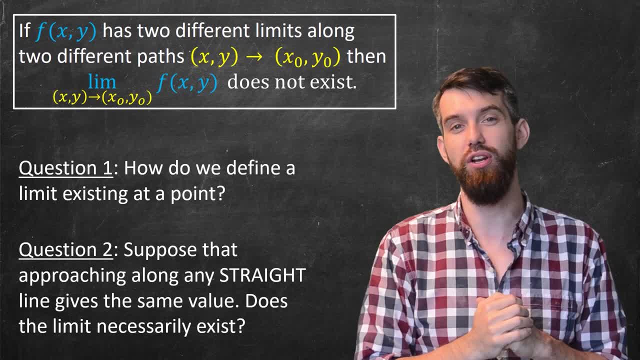 something else? or does all that matter? the straight lines again. a second question that i will leave you to think about for the future. if you have a question about this video, leave it down in the comments below. if you have a question about this video, leave it down in the comments below if you.